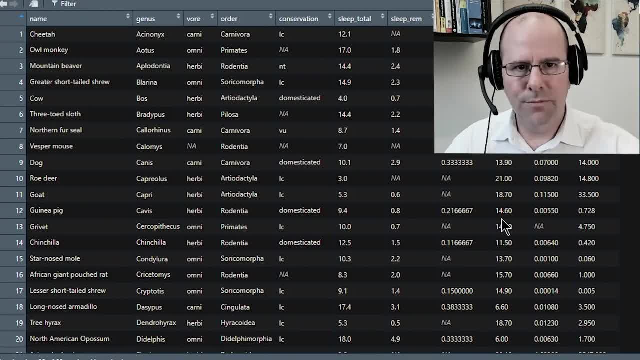 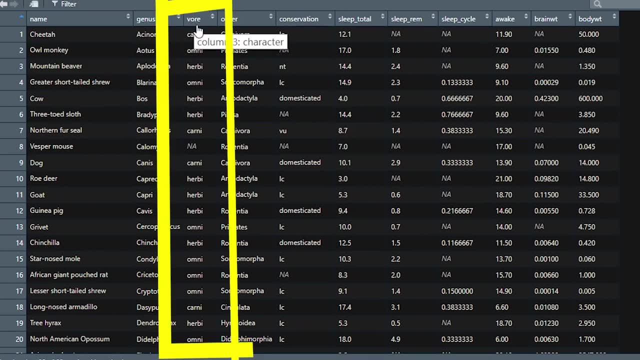 number line or categorical, which are categories, buckets. you can put the various observations into Right. so we've got numeric and categorical. Look, here's a categorical variable, for that's what these are all mammals, by the way, cheetah monkey, ba ba ba ba ba, Vore is what they eat: carnivore. 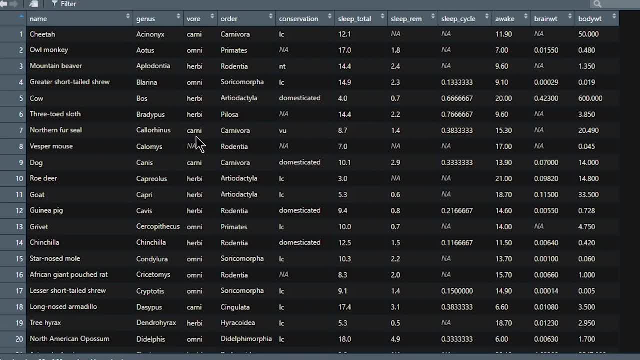 herbivore, etc. etc. These are categories. you can put each of the each of these observations or rows into and then look at this: total number, amount of sleep, total amount of time spent awake. these are numeric variables, Right? so we want to know how it is that we can create a graphic. 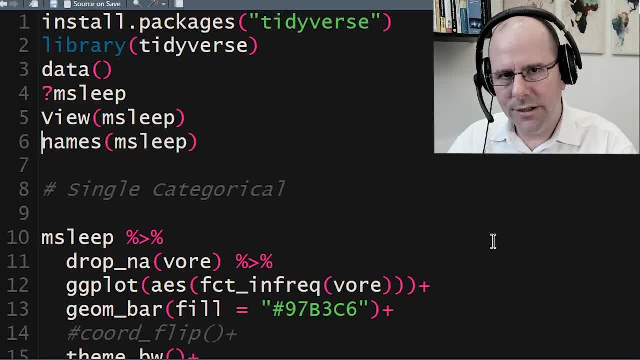 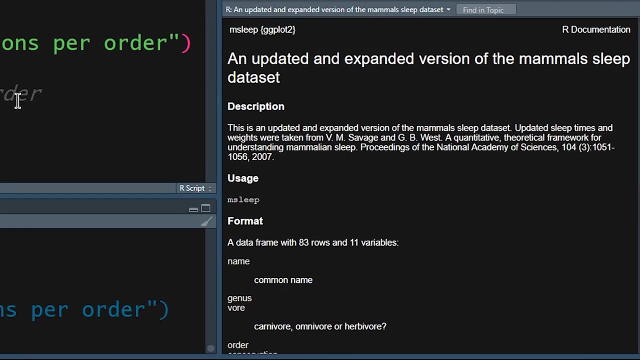 that takes into account information about both a categorical and a numeric variable in the same plot, Right, just to recap, right, I'm going to do a really, really fast recap of how we got to this point. If we have a single categorical variable, like we're just looking at herbivores or the vores, 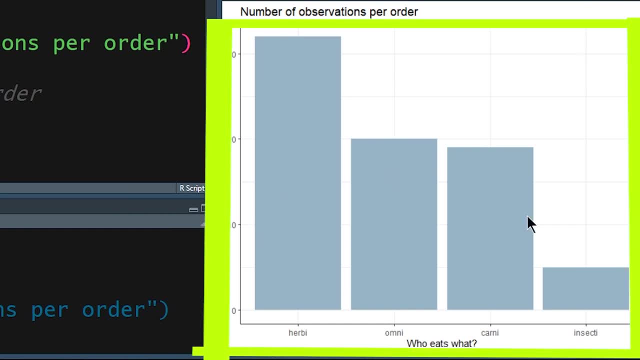 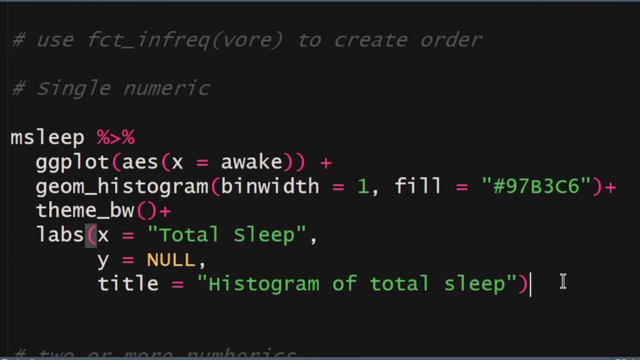 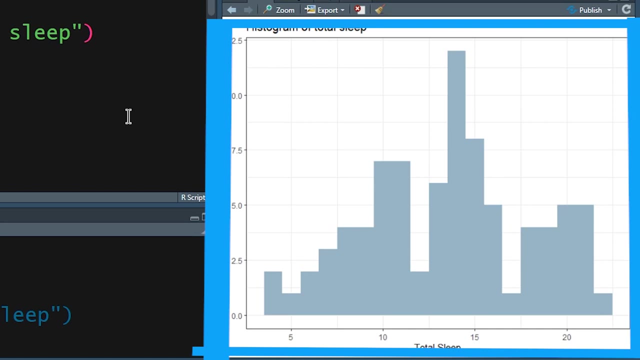 and we have a number line variable, then we create a bar chart counting up the number of observations in each category. If we look at a single, just one variable, which is, if we just look at a single numeric variable- okay, so a number line variable- then we put, we create bins and into each bin we 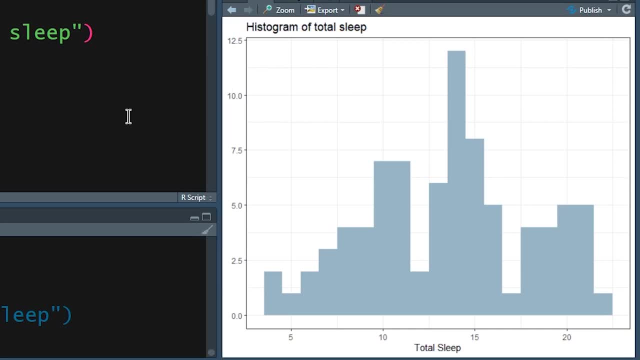 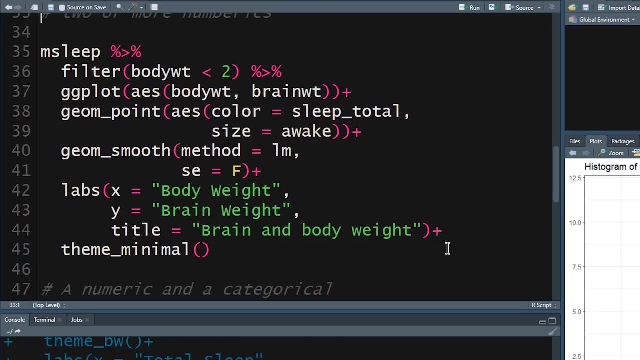 put the number of observations that fall within a certain parameter and we create what's called a histogram. So single categorical bar chart, single numeric histogram, Two or more numerics- we did this in a previous video- so two variables that land on the number line or more, and you 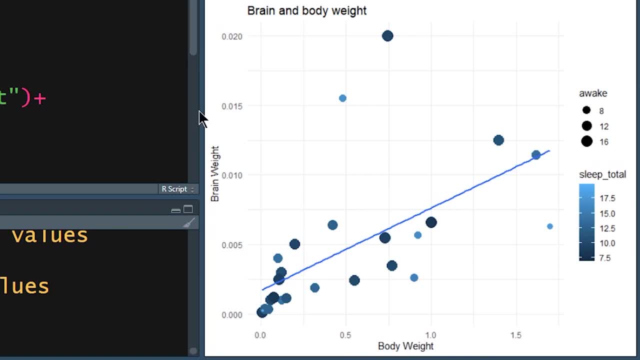 land up with all sorts of nice graphics like this where both the x and the y axis- here on numeric variables, we do a dot plot, we can draw a line through it, we can add other characteristics also, in this case numeric variables, mapping out against these data points. Not talking about that. 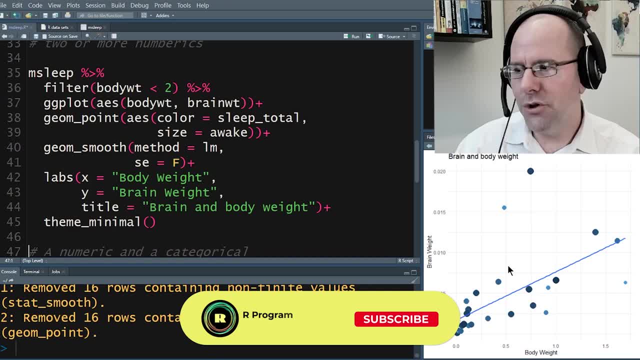 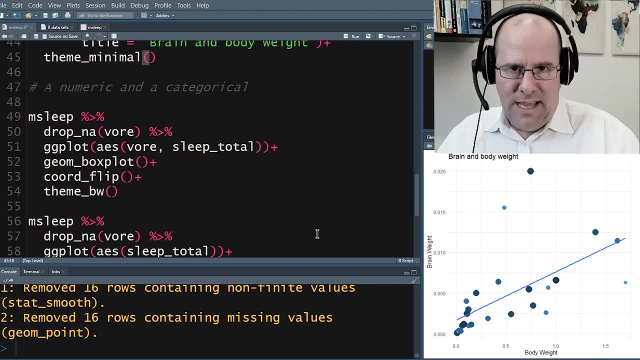 in this video. this is all a previous video. if you don't know what I'm talking about, go back and watch those videos. we're moving forward because today we're going to talk about a numeric and a categorical right. so in this case, let's say the total amount of sleep that a mammal gets, and 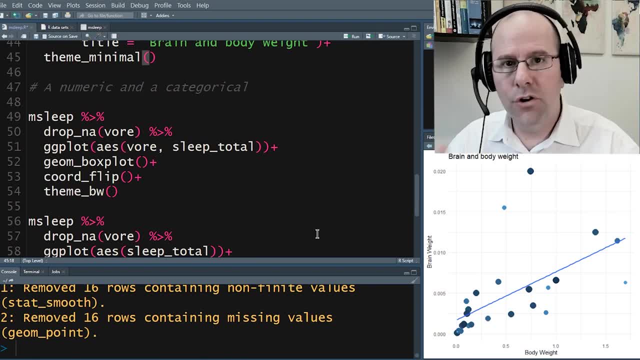 what kind of mammal it is in terms of what it eats. is it a carnivore, a herbivore, an omnivore, etc. etc. how do we graphically represent both of those ideas on one plot? and there's more than one way to do it right. let's get into this, okay. as always, I always suggest that if we're going to be using 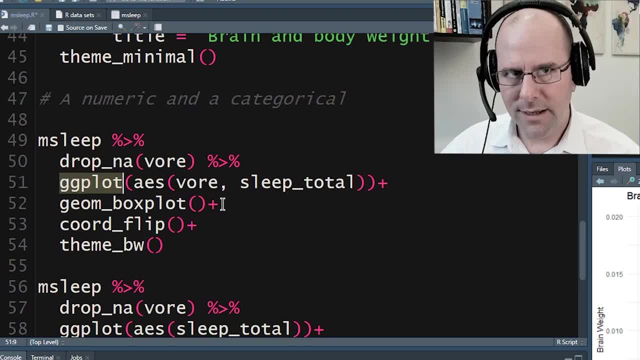 ggplot right and with ggplot, another quick, a quick revision. with ggplot, the three important factors that you need to, three important aspects of the plot that you need to always remember- and if you get this right you can do anything with ggplot- is: first of all, you tell it what data you're using. then 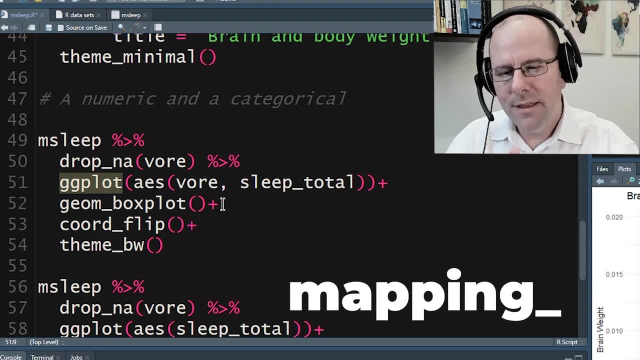 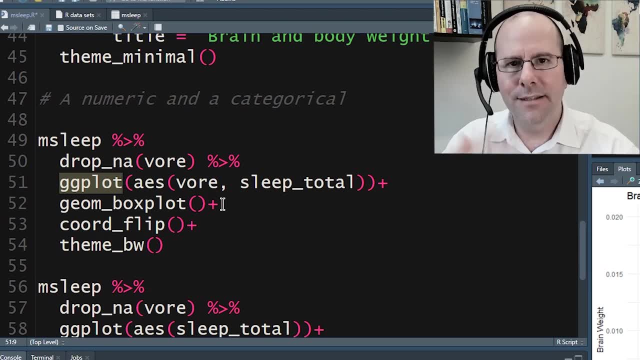 you tell it about the mapping right, how to map the particular variables against aesthetics, the visuals on the canvas, right. so size, shape, color. so you're going to say this variable must map out against size, this variable must map out against color. and then, once you've told, 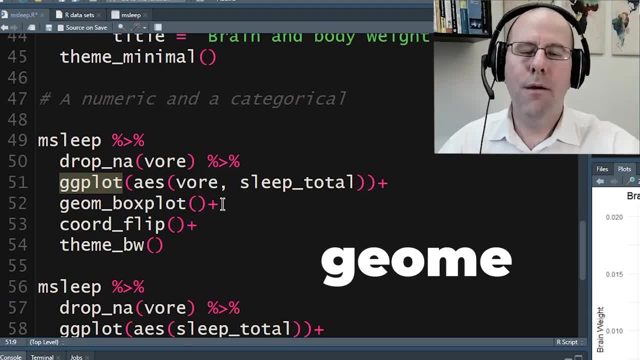 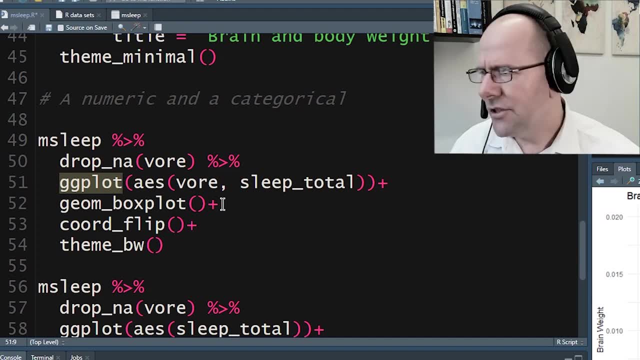 that information. you simply tell it what geometry to use- bar chart, histogram, line chart- you just tell it the geography and that mapping will just fit into place and it'll be magic right. so those are the three things. it's the data, the mapping and the geometry we ordinarily 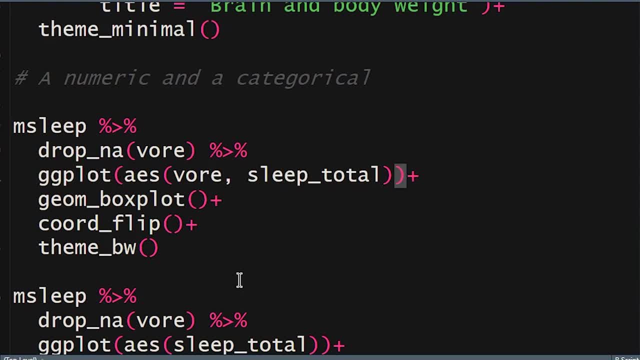 with ggplot you. the first argument you would ordinarily say: here data equals. we don't need to in the tidyverse, we can pipe data in, right. so we start off with our data set and this is the pipe operator. we pipe it into the next line of code and in this particular case, 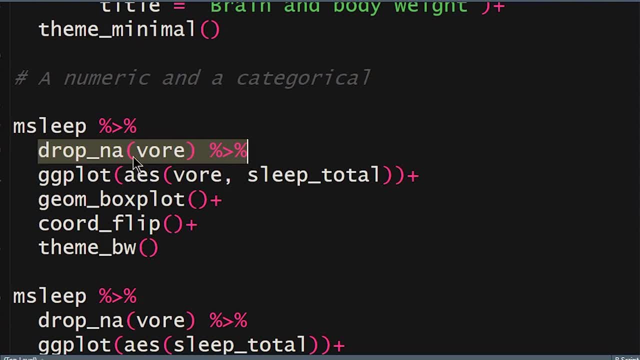 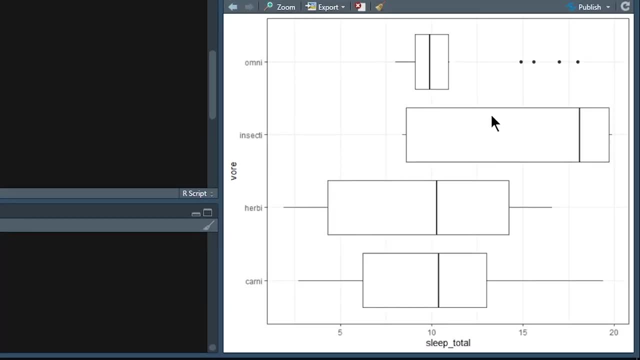 i'm saying let's drop the nas, which are the not available data points, from the vor variable. just to show you what i'm talking about, let's run that code, let's draw that plot here. so what we've done here- just to go ahead a little bit- is we've drawn a box plot, right, and i'll come back to the code. 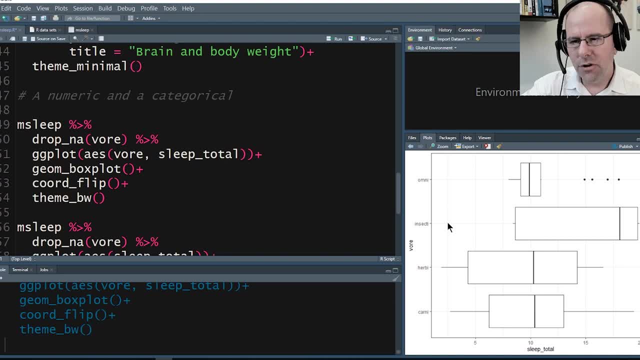 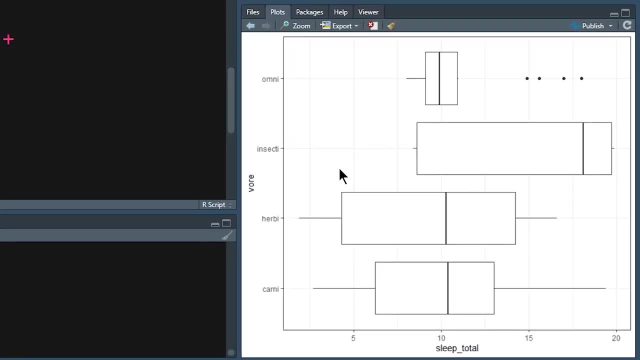 and talk about how we got there, but i just want you to understand conceptually what it is that we've accomplished, and then we'll come back and look at the code and see how it is that we how we got there right. we've got a categorical variable here: omnivore, insectivore, herbivore, carnivore. 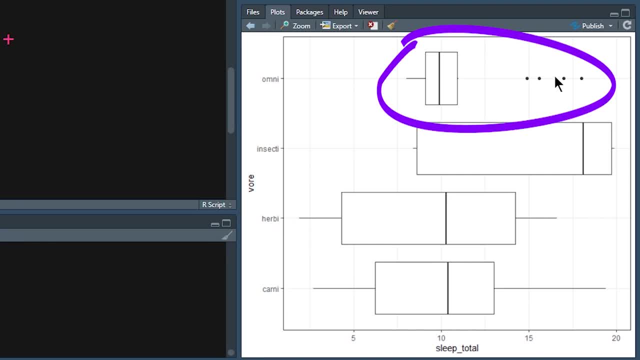 these are categories and within each category we've asked for the distribution of the values for this other variable, total sleep. so for omnivores, the total sleep values. now let me just quickly tell you how a box plot works. the box itself, this big box, contains 50. 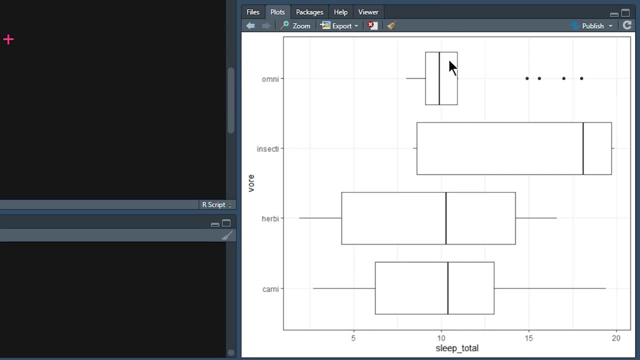 of all of the values. so half of all the values sit in the box itself. this middle line, the thick line in the middle, is the median. so that is the value which splits your entire data set in half. okay, the whiskers. see these whiskers here. they extend out for 1.5 times the interquartile. 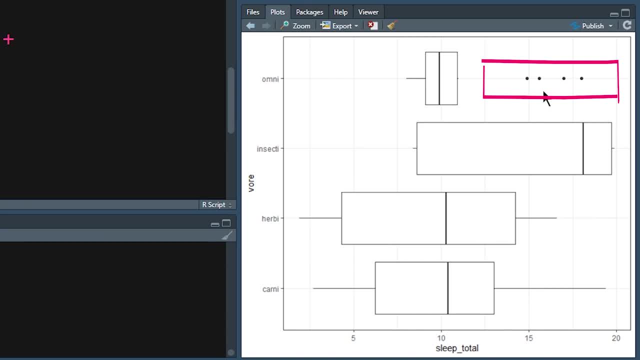 range, and then the dots outside are the outliers. okay, so that's just essentially. what you need to know is that this box plot is a representation of the distribution of this numeric variable, how the starter is distributed, and we've divided it up into by this, these categories, which are the values. 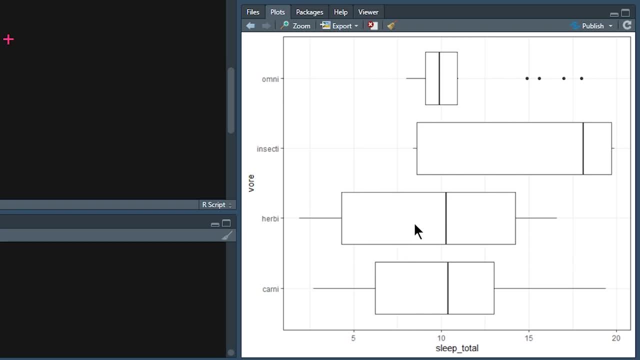 that are in the categorical variable. so that's, this is a nice example of in one visualization. we're visualizing both the numeric and a categorical variable in one graphic. now i haven't put on, changed the labels and put in the heading, etc. etc. we've seen that in other videos and i want. 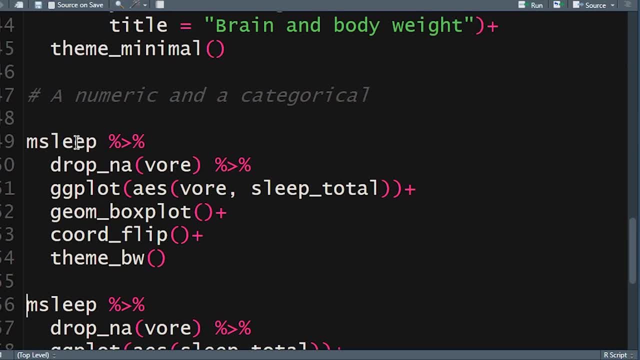 to get into that now, but i want to get into that now, so i'm going to go ahead and show you how this works. let's go through the code and see how we got here. we started off with mc. that's our data set. we've piping it in to ggplot, but the reason using these pipe operators and piping the data in is 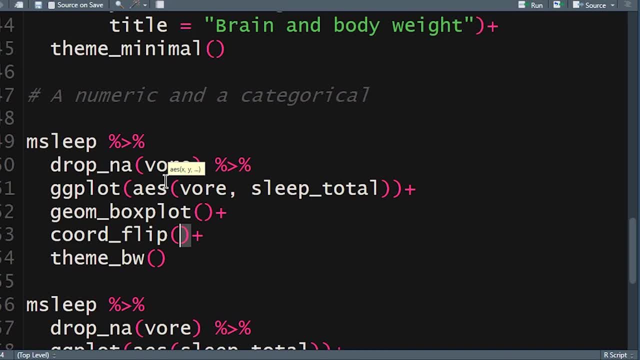 powerful is that you can make changes along the way. in other words, we can. we can manipulate the data so that what gets piped into ggplot is exactly what we want. and that's what i've done here. i've said: drop na. let me show you what happens if i didn't have that line of code. 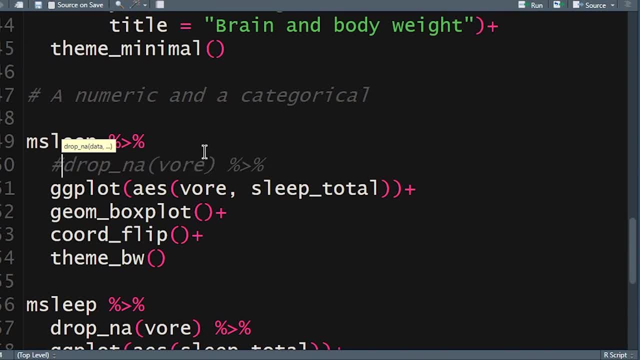 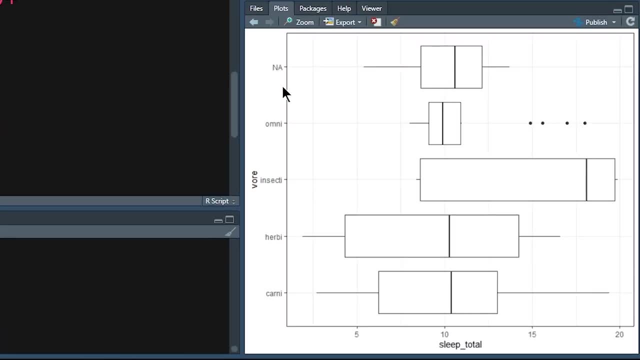 and to do that, i'm just putting a hashtag in front of the drop na, which means that r will ignore that line of code. it'll just run right past it and if we run this chunk again, you'll notice that now there's an additional category called na. in other words, this is the distribution of data for which there was no 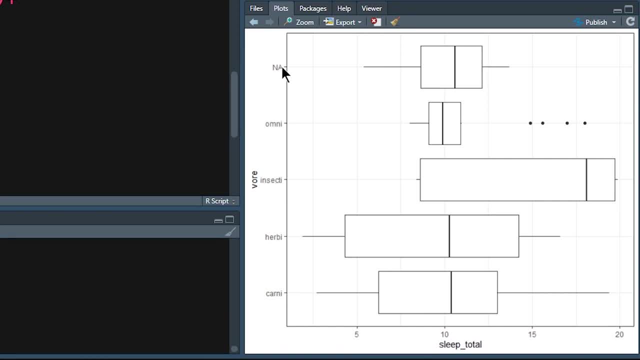 indication in the data set as to what that particular mammal ate, and so that data point was not available. with respect to the categorical variable and the distribution of our total sleep in that new category of na is, you know is is represented here, so we might want to say: look. 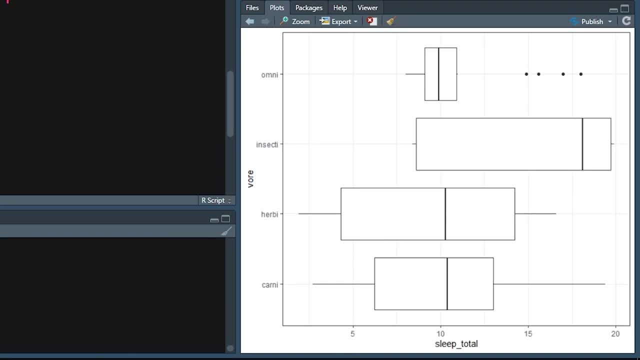 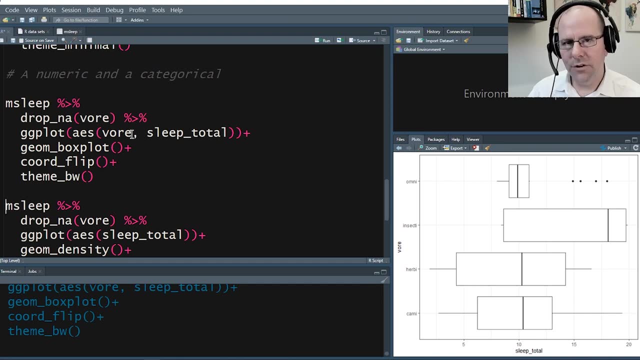 we want to drop those na values and just look at data where we do know what the animals ate, and there we go. so that's the power of using the pipe operator. we manipulate the data on its way to ggplot. it gets to ggplot and because we're using the pipe operators, the first argument 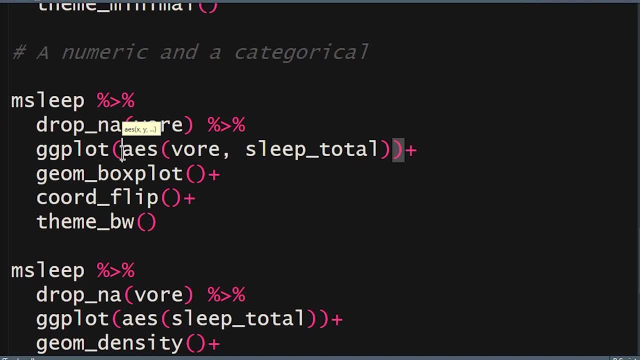 in this function is assumed to be this data frame getting piped in, so we don't need to tell ggplot what data to look at. the first thing that ggplot wants to know is the mapping. right now we could say: mapping equals aesthetic. we're going to say: mapping equals aesthetic. we're going to have to. spell mapping, which is the file nam and ge leafing log. it does. that makes sense. so now we need a some olmak alpha and after typing and pasting we're going to need a mentor and a mk 그러� to analyze what data is. we need to take that map키 to find and help let us plot and determine what we want to do. the mapping here. 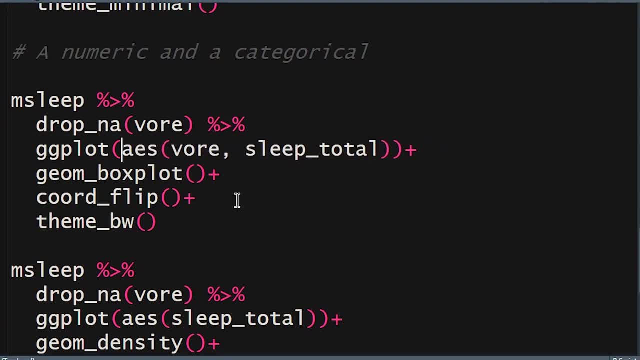 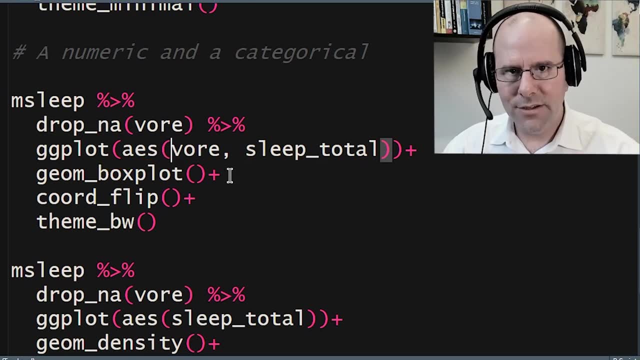 quills aesthetic. we don't need to. gg plot knows that that's what we're trying to do. when we say aesthetic, we're saying all of these aesthetics, that the visual aesthetics, color, size, shape, axis, etc. etc. what are they going to map out against with respect to our data frame? r assumes that. 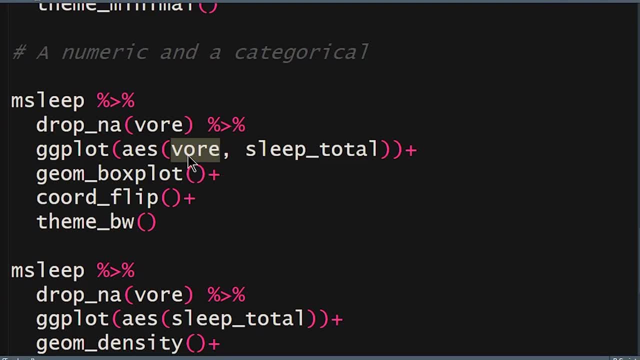 the very first piece of information within the aesthetic is the x axis and that the next one is the y axis, and then after that you need to tell it color equals, or you know. you need to actually be a bit more specific. now you'll notice. you may be a little bit surprised because you might say: 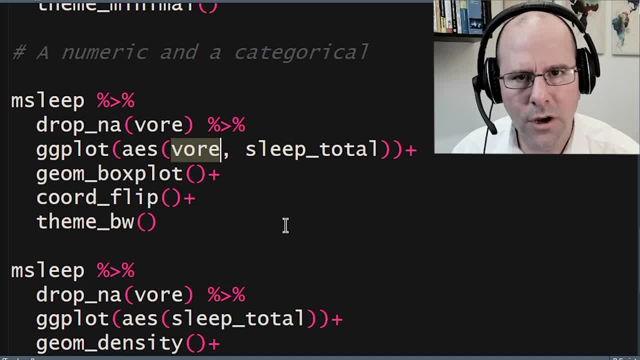 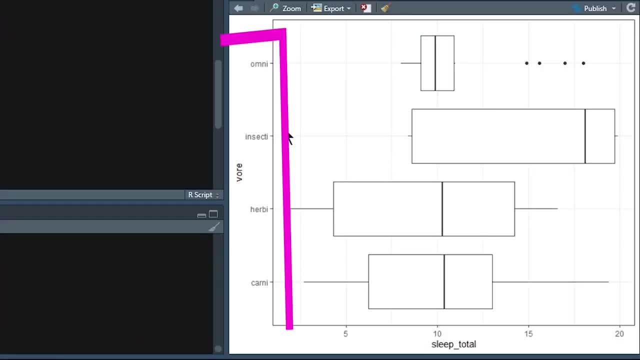 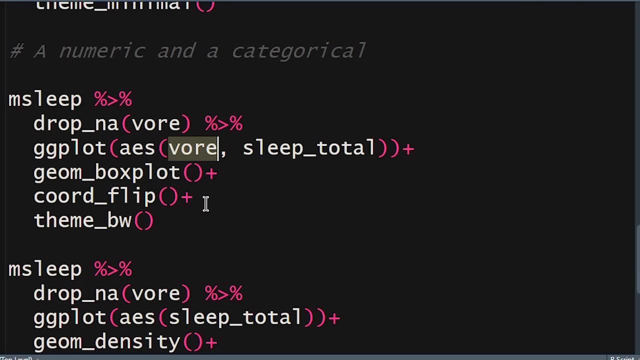 well, greg, look here you've got vor in as the first argument. you've said that the first argument will always be understood to be the x axis, and yet here on your actual graphic, vor is clearly not the x axis, it's the y axis. well, nobody panic, that is because down here i've said: co-ord, flip right. 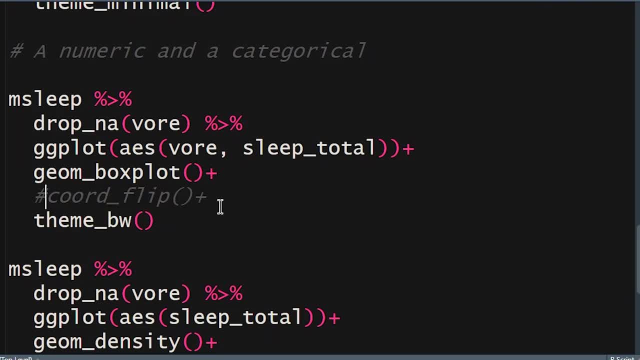 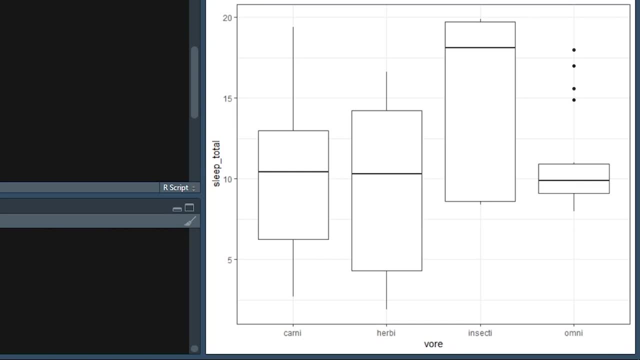 so so if i just just that we we don't get confused, i'm going to tell r to ignore code flip for now, so you can see exactly what i mean. okay, without the code flip command right. vor is our x axis down here. vor is our x axis and the x axis is our categories. total sleep is our y axis and it's got. 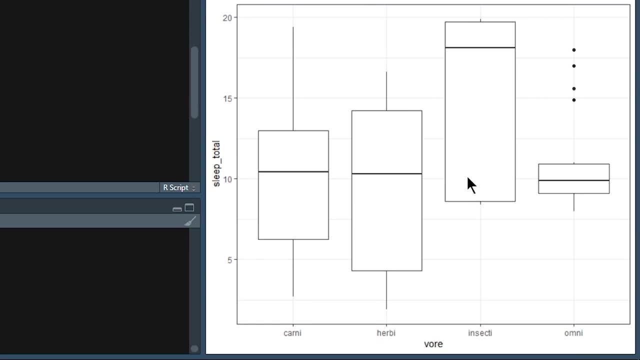 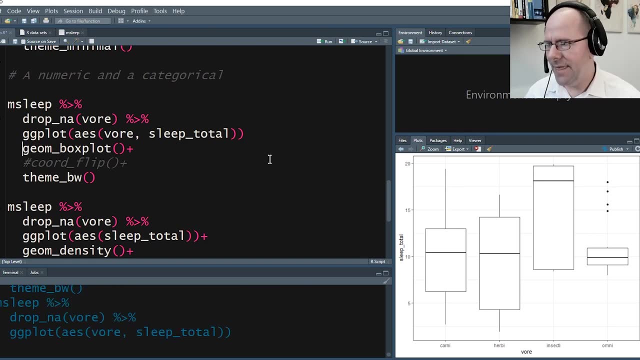 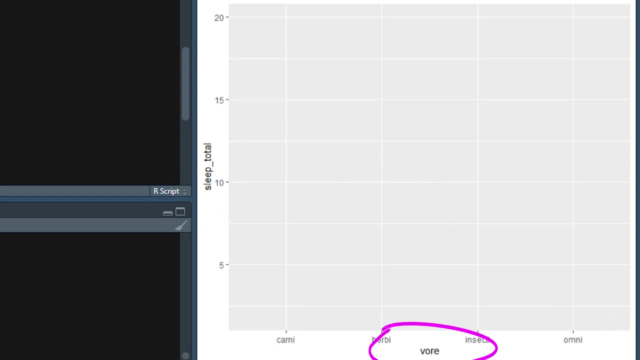 the distribution of that continuous or that numeric variable being just being represented. well, at this point it's not being represented by anything. if we take away that plus and we just ran that code. look, here's a piece of canvas and you've told me that sleep is y and vor is x, but i haven't got any geometry to. i don't know what to do with. 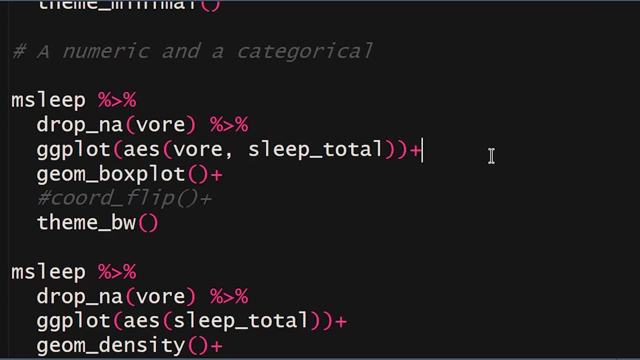 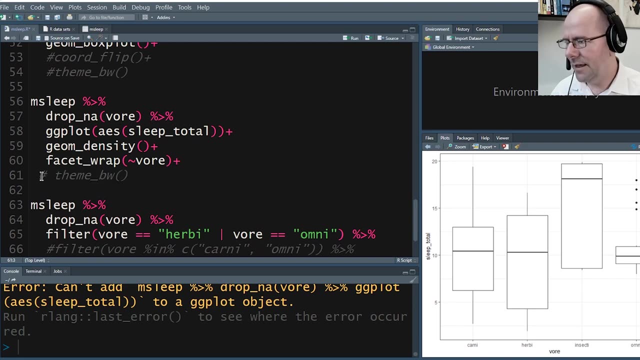 that. so we put in a plus and then we put geom box plot, right. so we're telling it the geography to use and voila, there's our box plots theme. i've just said, look, if i don't put that theme in there, it's gonna, it's gonna use the default theme if i put in a hashtag there and removed that plus. 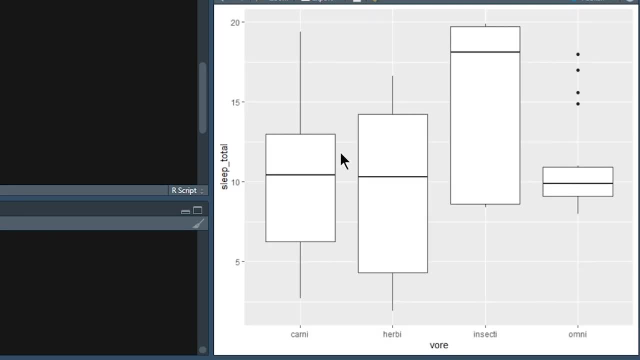 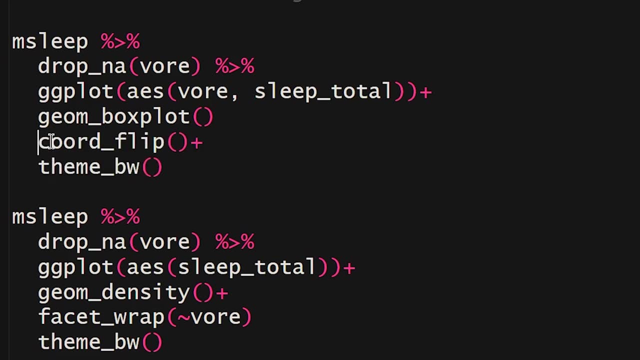 okay, here i am. if i remove the theme, it goes to the plus and then i put in a plus and then i put in a default theme. i prefer either the black and white or the minimal theme and, and when it comes to box plots, i prefer to include the code flip and i'll tell you why your box plots when you're mapping a. 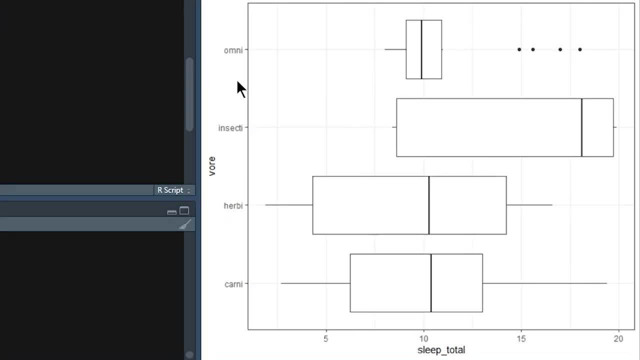 categorical and a numeric variable. your categorical variable is usually words, while your numeric variable is usually numbers, and the words can be kind of quite long. if these are all on your x axis, those words all have to be written, kind of, either at some sort of strange angle or 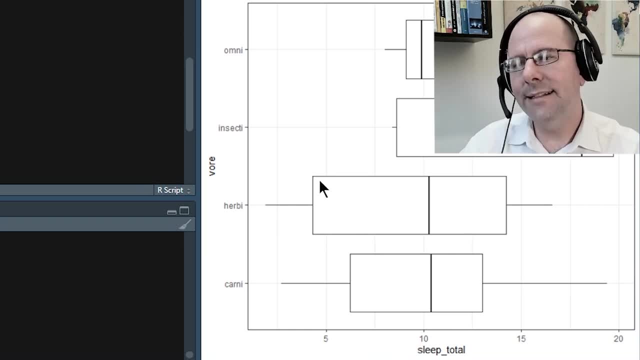 at like 90 degrees it gets a bit messy, whereas if it's your y-axis they can all be written sort of horizontally and they're easy to read. so i much prefer doing a code flip if i'm doing a box plot that involves a numeric and a categorical variable. right now, let's start. 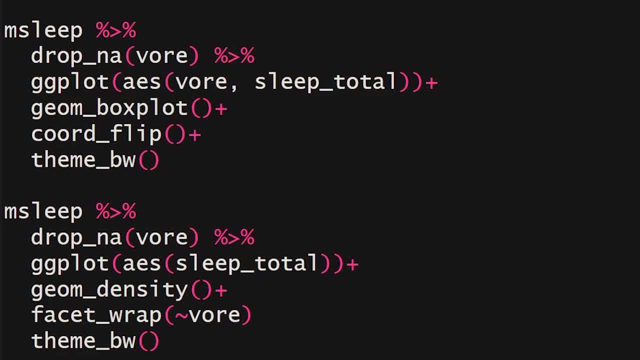 looking at other ways that we can represent the same kind of data, right? so we look, we're talking about a categorical variable- omnivore, carnivore- and we're talking about a numeric variable- total, sleep. right, we've got some more code over here. we've got the same, the exact same principle. 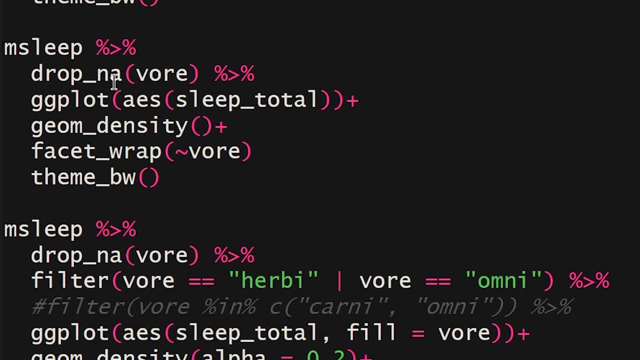 applies m. sleep gets piped into drop nas. all the missing values from vores disappears. gets piped into gg plot. and here i'm just defining the aesthetic as sleep total and i'm asking for a density plot. and then i'm doing a facet wrap by vore. let me run this and then go through it. 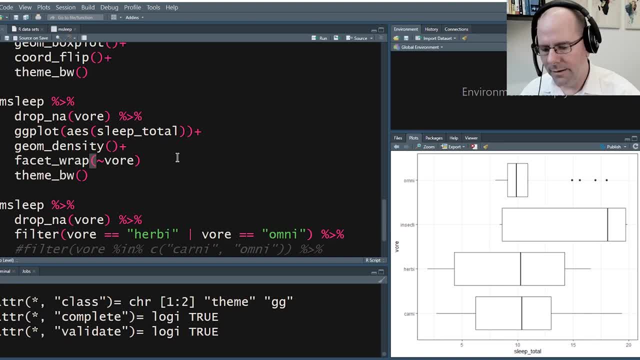 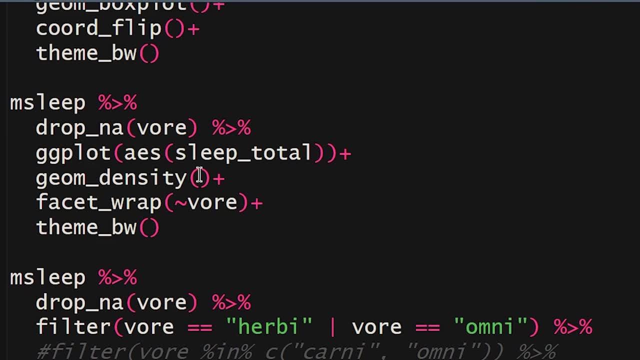 a little bit more carefully and you'll see what i mean. okay, sorry, i need to put in a little plus over there. okay, let's go through this one at a time. and actually you might understand this a bit better if we change this to geom histogram, because that's something people are familiar with and we've 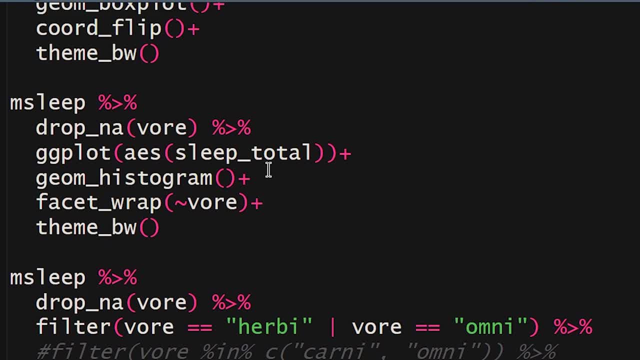 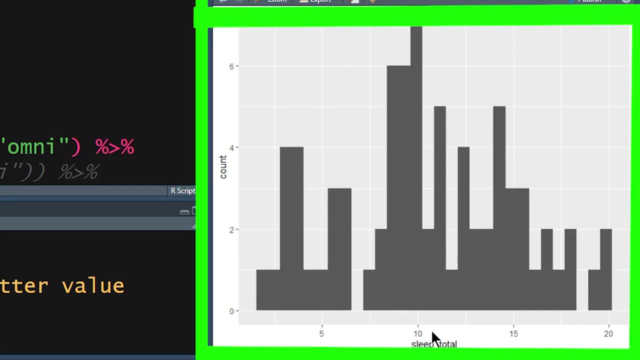 already talked about that before. okay, and let's not do the facet wrap yet, so we're just going to stop right there. if i ask r to draw a histogram of of all of the total sleeps, it'll, it'll. just. we've talked about histograms before. you know. you understand what this is. it creates bins. 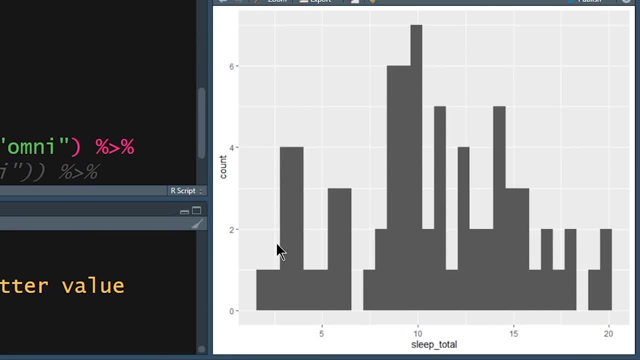 it looks at any given data point or any given row or observation and decides which bin that goes into. these bins get in the context of the histogram. so we're just going to go ahead and do that and then we'll get on together for a while. so we go through it as one and then we'll work on this. 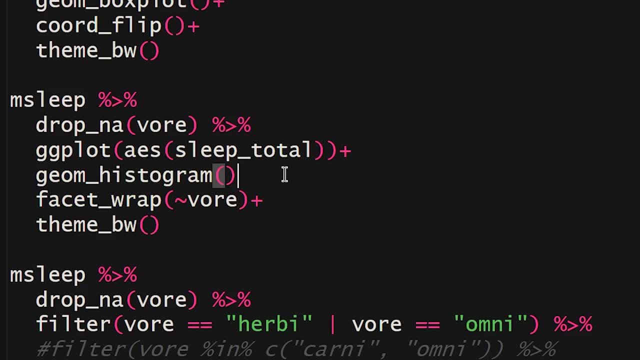 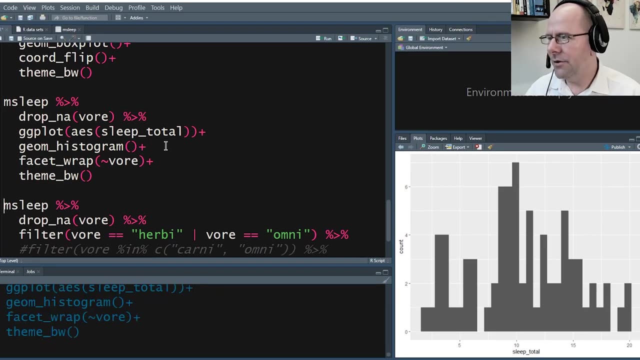 to get along again. good, it works in very similar ways as fine. but what we're about to do second is look at geographical distribution, because this is a little more interesting when we compareór of the histograms, because we already have a nice policy to eliminate sóc and we might now want to say, well, let's divide that up into separate graphs and each graph looks: 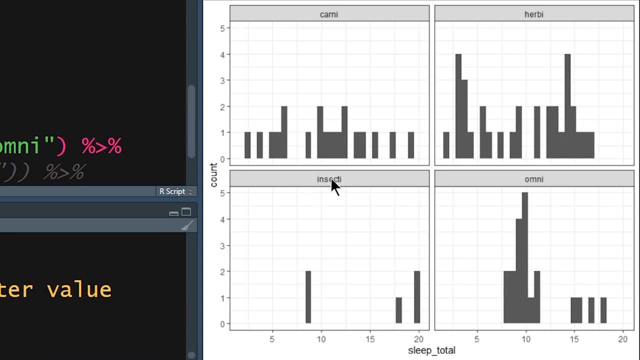 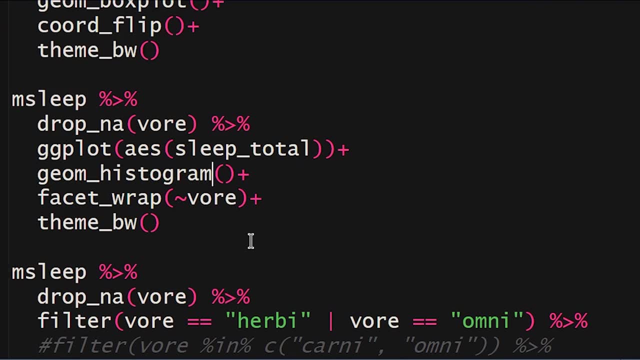 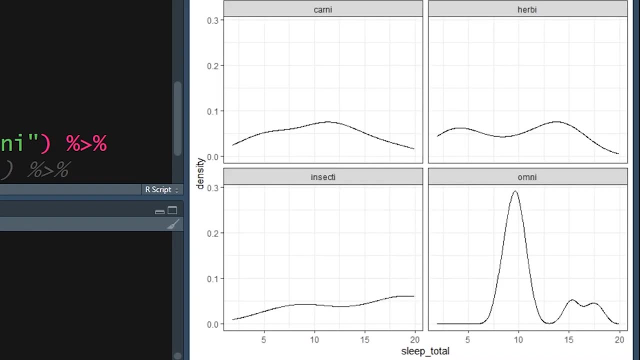 at only the data that is associated with a particular category, and so now we run the data right and that's fine. so you understand a histogram, a nice way of representing this is, instead of a histogram, a density plot. and what a density plot is a density plot is it's exact? 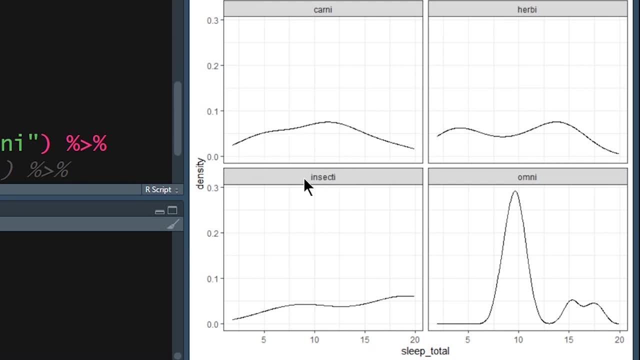 same idea as a histogram. right, it's looking at the shape of the data, the distribution of the data, but instead of actually counting up the bins, it looks at: at any point along this number line, what is the probability of a value being at that point? and probabilities are between zero and one. so the 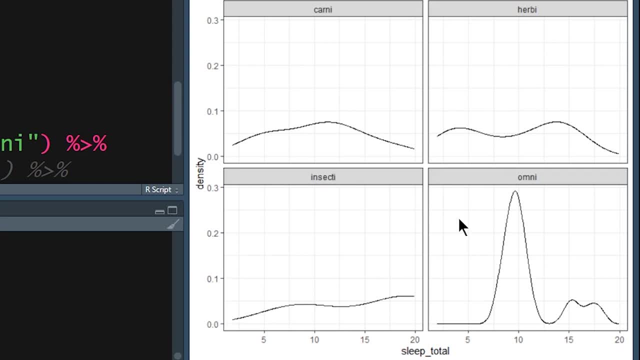 density plots are always these kind of fractions between zero and and the highest value. here is point three, but it can't go higher than one, right? so? so that's how density plot works. they're kind of nice, they're easy, they're very intuitive. when you see a density plot it's very easy to kind of. 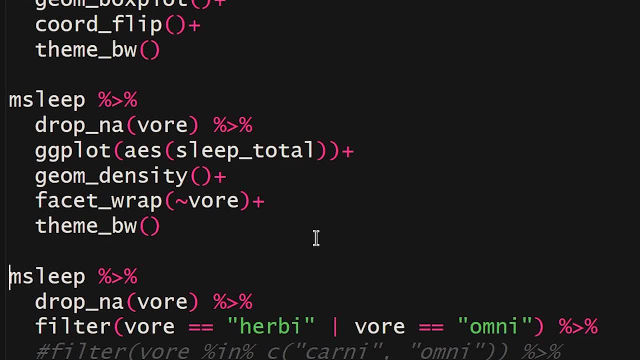 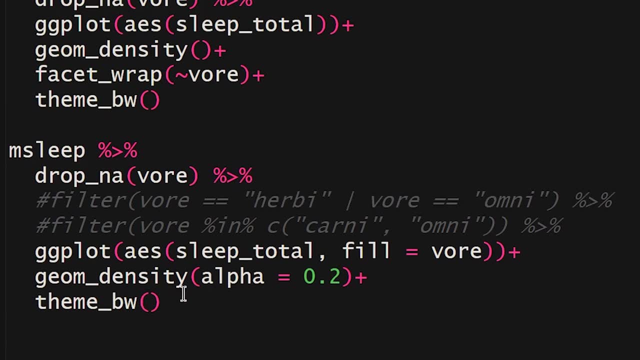 understand what it is that it means. now i'm going to take this idea of a density plot one step further. okay, and i'm going to run a density plot. instead of using the facet wrap and putting it into four different graphs, i'm going to layer the densities on top. 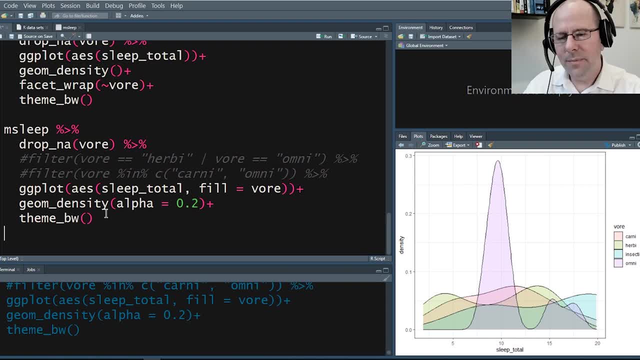 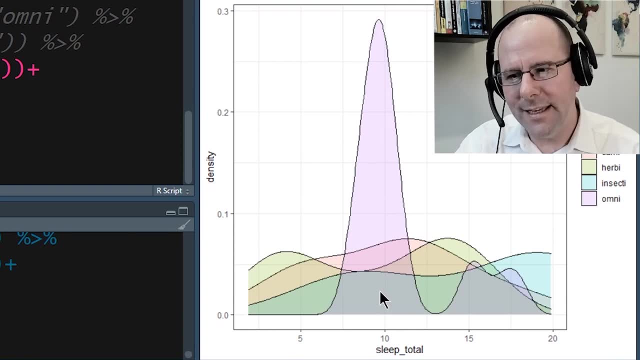 of each other and give them a color which is kind of quite nice as well. but there's a caveat. look at this particular graph. it is nice, it looks kind of nice, but it's a little bit too busy when you've got four things that are kind of quite similar all layered on top of each other with a 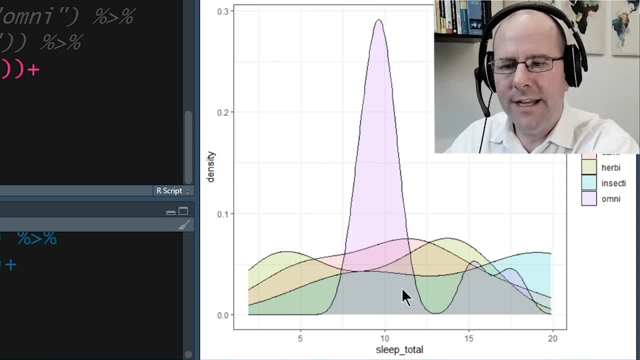 color. it becomes a bit too busy and it's a little bit messy. it's difficult to tell exactly what's going on there. so under these circumstances i wouldn't recommend using a density plot, because it's a little bit messy and it's a little bit messy and it's a 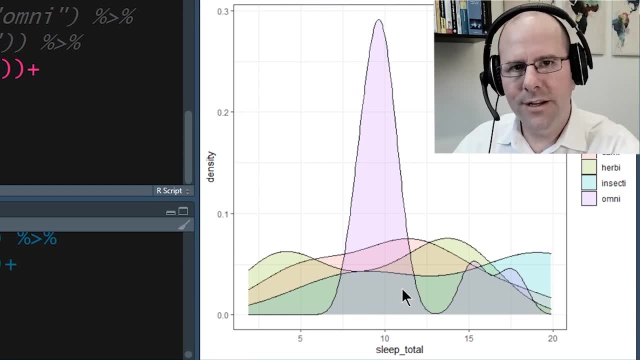 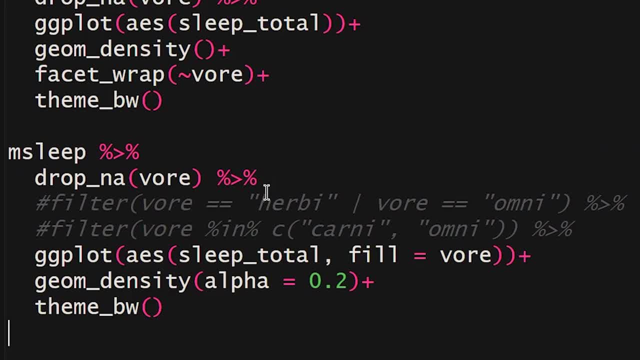 times when it is kind of quite useful to do right. so ignore these filters. i'm going to bring them back in a sec. i'm going to show you a couple of tricks. same story: m sleeps our data pipes into drop na. we're removing all the missing values from the vor variable. we're going into gg plot. we're. 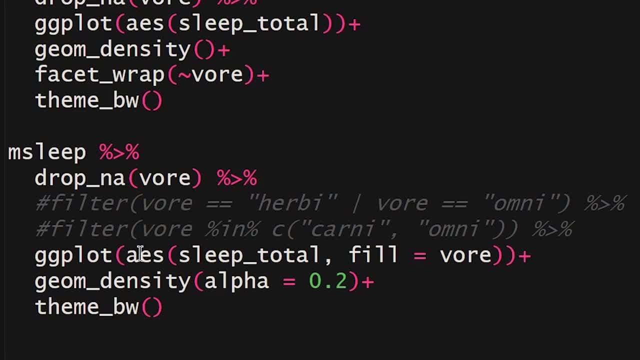 saying we know what the data is, but the mapping is going to be against the using the aesthetic total sleep. and then here's another aesthetic. we're going to say fill equals vor. in other words, we're saying wherever it sees the variable vor, the different categories in that it wants to use to fill it up. 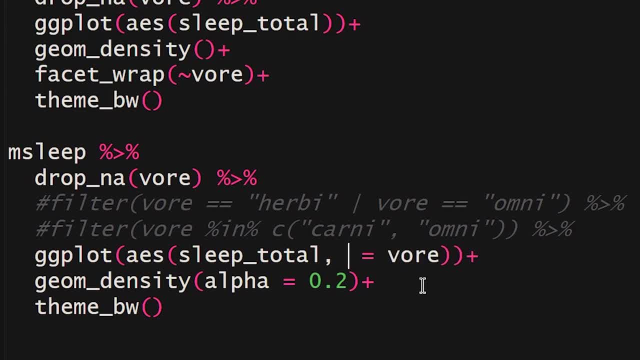 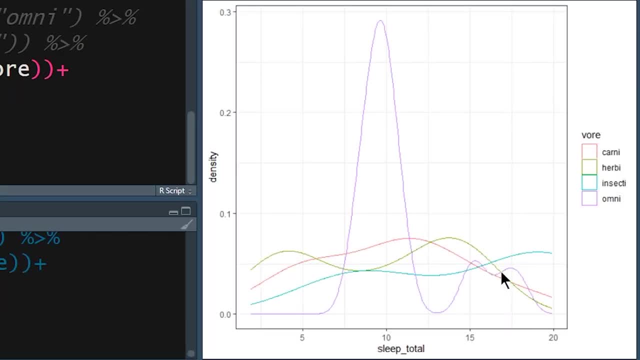 using a color. that that's for now, just that you know what i mean. if i made this color equals vor, it would draw lines and that's actually a little bit easier to follow. to be honest, that's a little bit easier. it would draw lines and but instead of color, if you said fill, 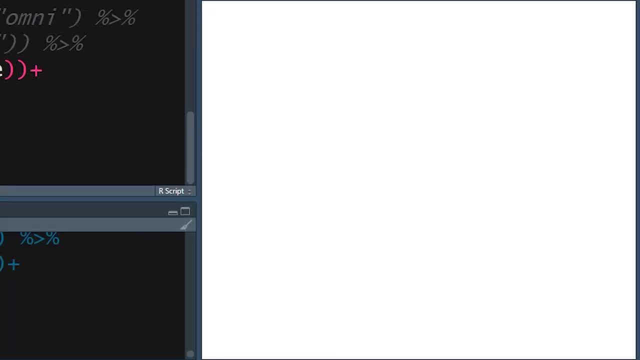 it filled, it would draw lines and that's a little bit easier to follow. to be honest, a lot of models that allow that. a little fairy tale. it might be the only way to do that too. i just want to show you an example, overhead and overhead. so you need to go above what? 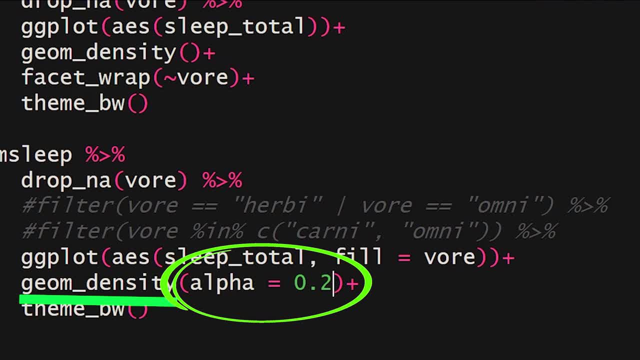 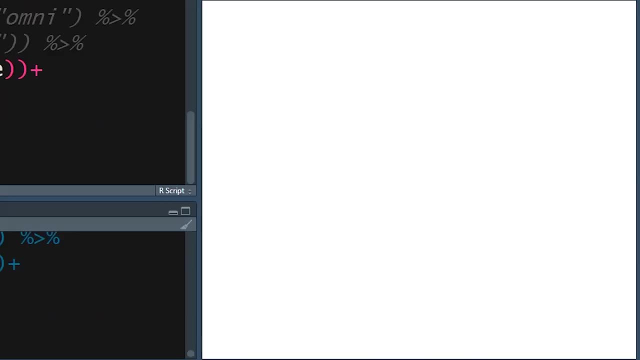 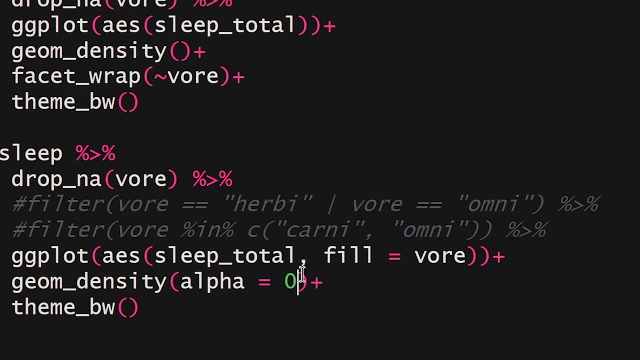 that row, which is this line, through that you know the, and it's difficult to see what's going on. sometimes that's actually easier if we said alpha equals, you know, 0.3. it makes it a bit more transparent. if alpha was equal to naught, it would be completely. 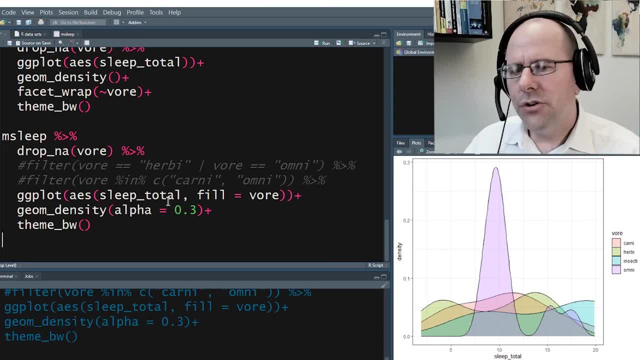 transparent right and theme black and white. that just makes this a little bit nicer. so that's the density plot. now here's the tricks that i want to show you. this density plot, we've said, is a little bit busy. we've got four different layers, one on top of each other. it's a bit difficult to see. 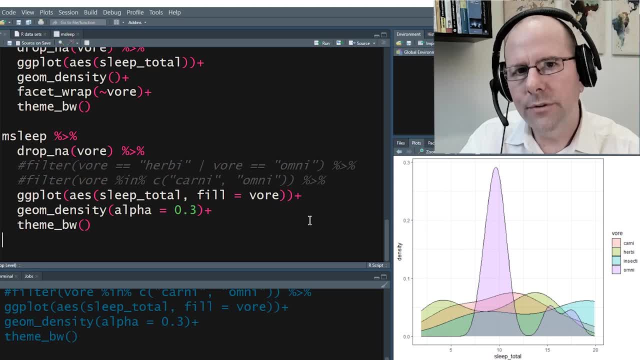 what's going on. these layered density plots are kind of useful when you have fewer categories. so let's imagine that we just wanted to use two of these categories instead of all four. we wanted to use two. that would mean that- and this is another reason why this piping is so powerful- 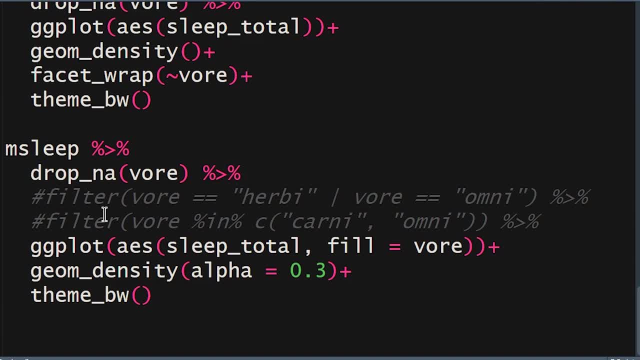 we want to pipe a data set in that gets filtered and extracts only out the data that we want, and that's what gets used by ggplot. so let's look at the first example of how i've done that. i've said: drop four is baba okay. 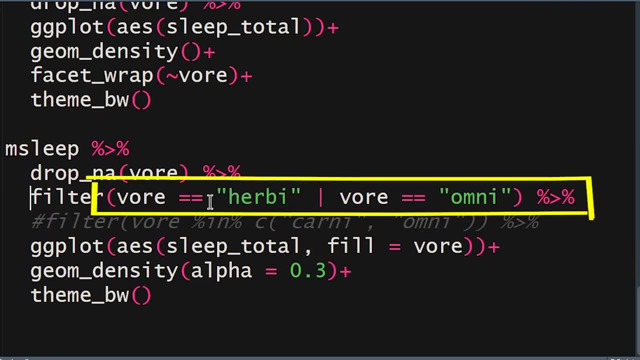 now let's look at the first example of how i've done that. drop four is baba. okay. now let's look at the first example of how i've done that. filter the data, and i've got two criteria here. one is that four is double equal to herbie. now 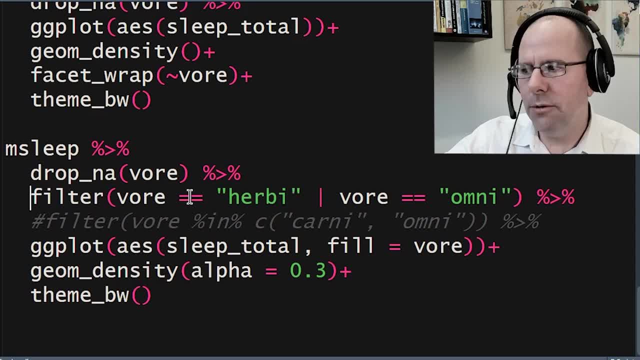 let's just talk about that for a second. what do i mean by? why have i got two equal two signs here? when you're using r programming, if you put one equal sign, you're telling r that what's on the left does equal what's on the right. you're making a statement: this is is equal to that. if you put 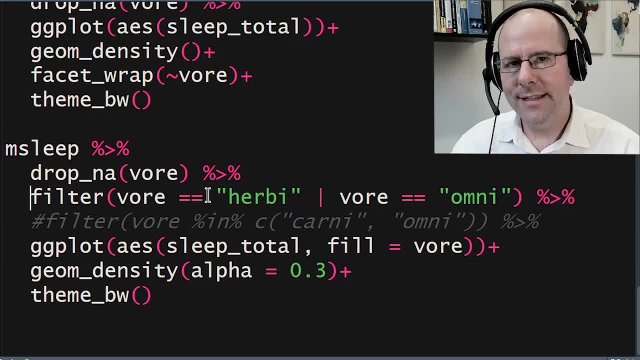 two equal signs next to each other. it's more like asking a question. it's saying: select the data where it is the category that you want to use, and then you're going to put two equal signs next to each temporal at that point and then you're selecting the top qР, that five plus X. 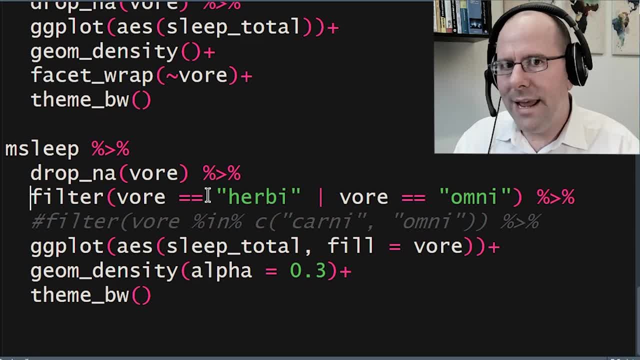 right. so it's more of a question. it's saying: extract data points wherever this criteria is met. wherever this is true, voor is equal to herbie, that statement gives us a true: we'll extract that row of data, and then the or that line there is is basically means or. 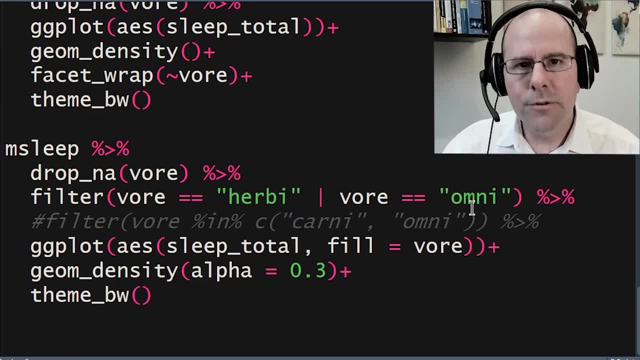 or if four is equal to omni, extract that as well. right, the difference between or and and. if that was an and it would be wanting both criteria to be filled before it extracted that row of data, and we'd get nothing. if you say, or it's like, if it's this, or. 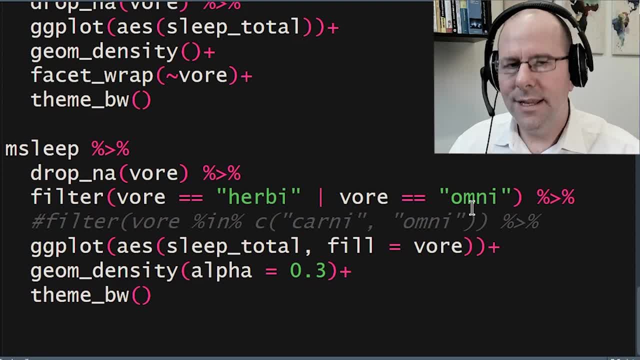 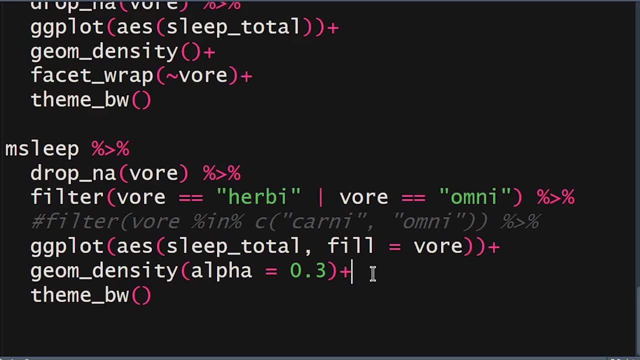 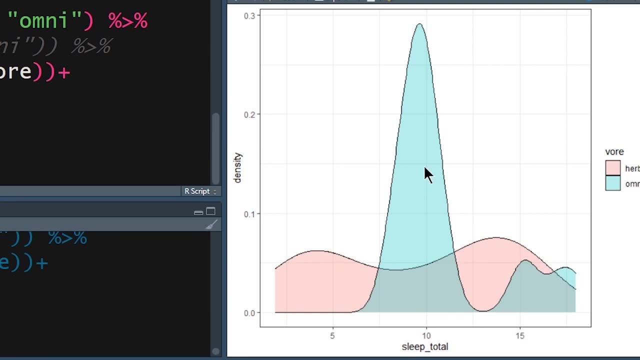 it's that if either of these criteria are met, then that's a row of data we want. if both of these criteria are not met, then then leave that row of data alone. so if we ran this, we would be just looking at herbivores and omnivores, and that's much easier to read. that's much easier to look. 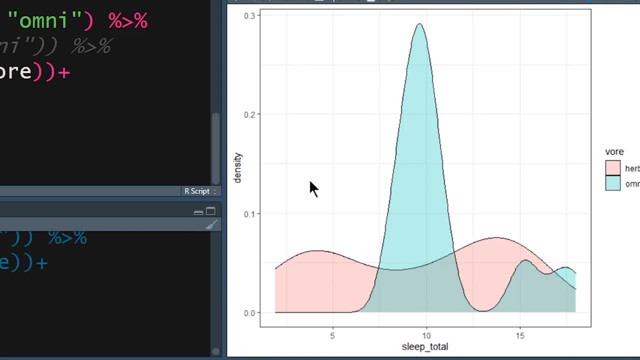 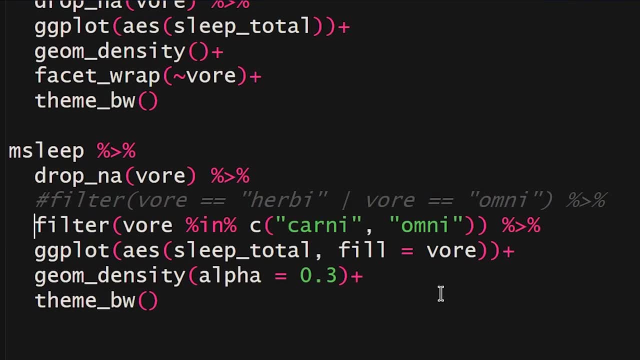 at right because, you know, even though they're overlapping, it's a little less messy, it makes a lot of sense. another way to do the filter, because i just sort of sort of think: well, while we're talking about filtering, what if we wanted we had more than just two? what if we had a whole lot? 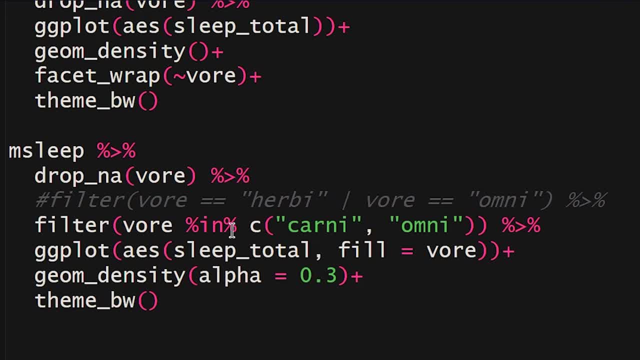 it becomes quite difficult to do this whole. or story r has got this little feature here which i like a lot. you can say in it's kind of like the pipe operator. but you've got a little in there and you're saying, well, we want to filter for any row where the vor in which the vor meets these. 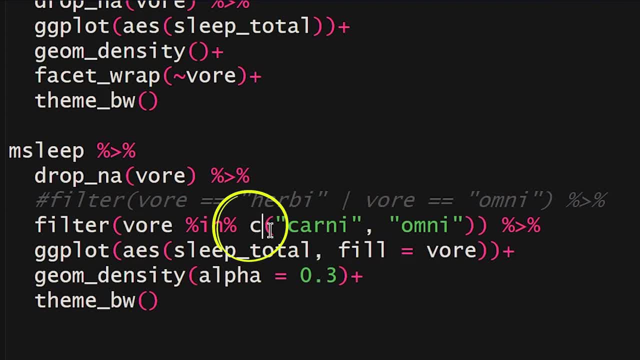 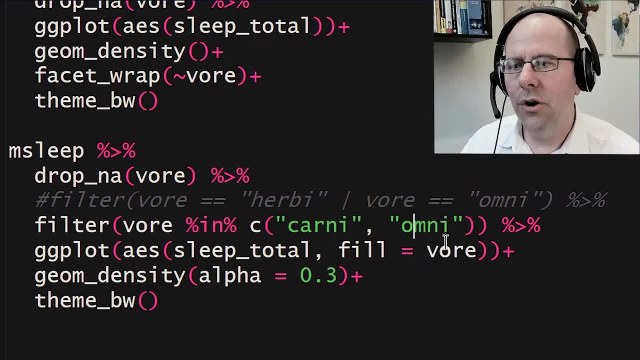 criteria? either of these criteria. so we're going to filter for any row where the vor in which the vor meets these criteria, and then you have a concatenation, open brackets and each of the criteria separated by a comma. when this becomes useful is when you actually have a whole long, long. 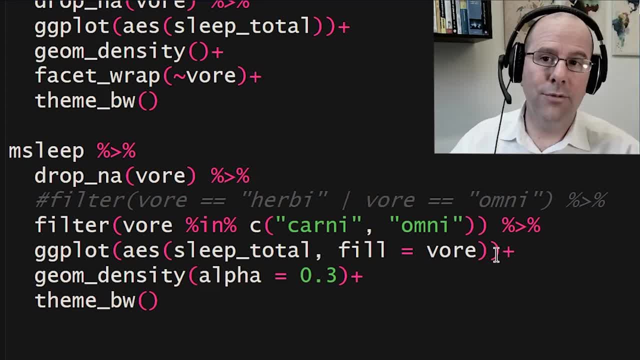 long list and you can just stick that in, or you can make that list into an object and pop that object in. it's a nice trick. once you start getting used to using that little in the story, you'll use it a lot. it's a big time saver, and so in this case we're looking at carnivores and omnivores. 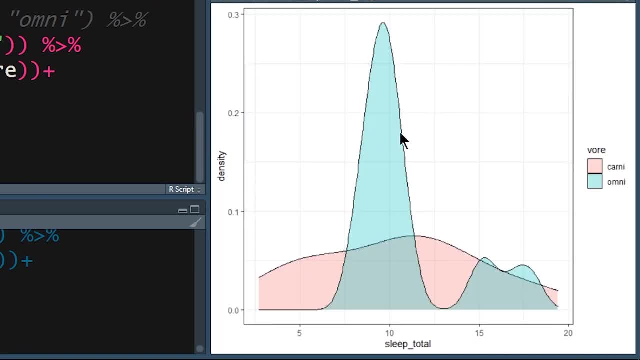 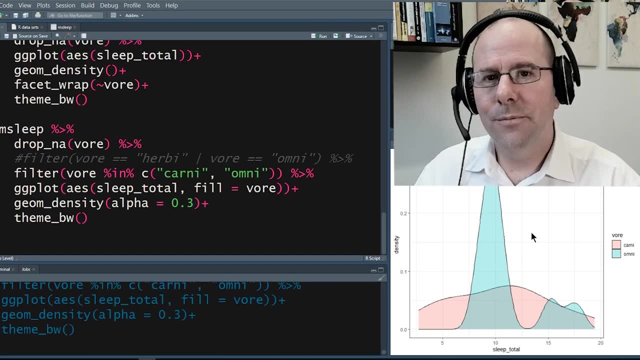 and you'll notice. voila, the same sort of thing happens here. we've got carnivores and omnivores layered on top of each other with a density plot. very, very nice. you've got to love it. you've got to love r listen if you haven't subscribed to this. 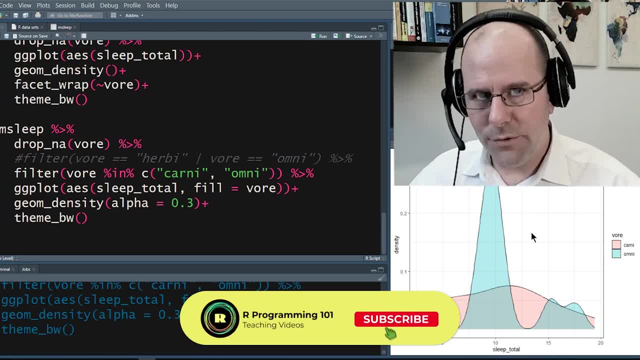 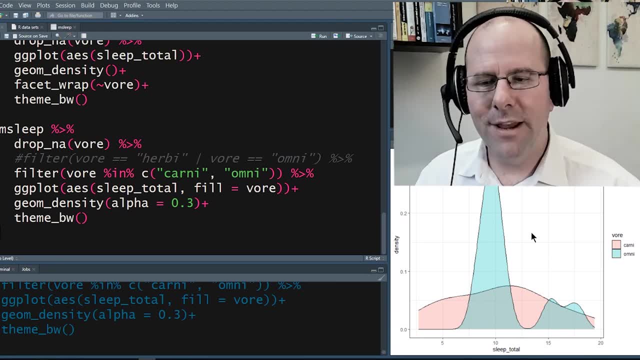 channel yet please do hit the subscribe button. hit the bell notification if you want to get notified of future videos. leave a comment below if you've got any questions, thoughts, if you just want to say hi, that would be great. share the video with others. hope you have a great day. don't. 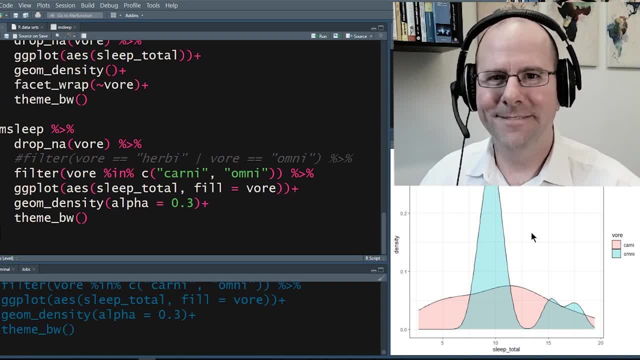 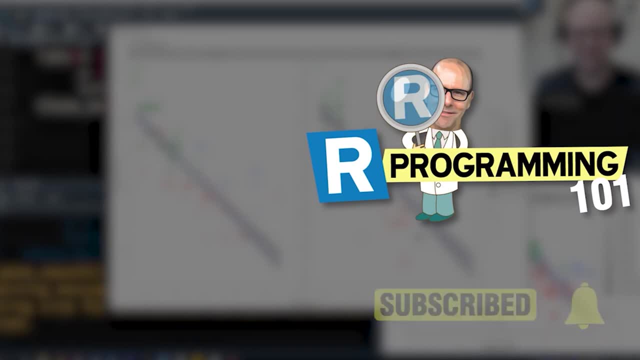 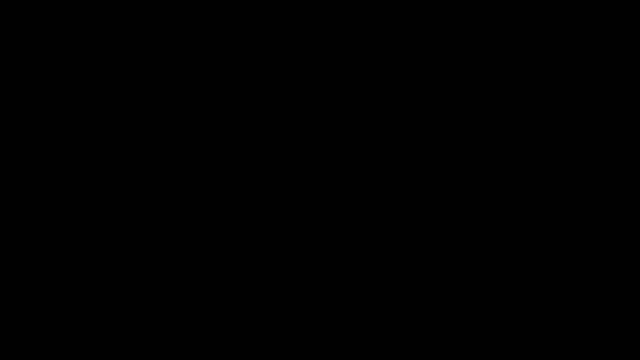 do drugs always. do your best to over change. speak to you soon. take care, bye, bye.